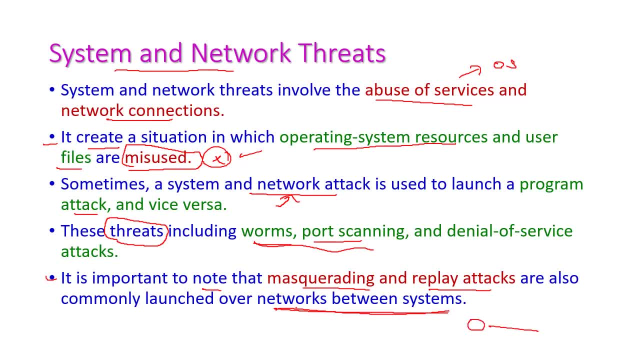 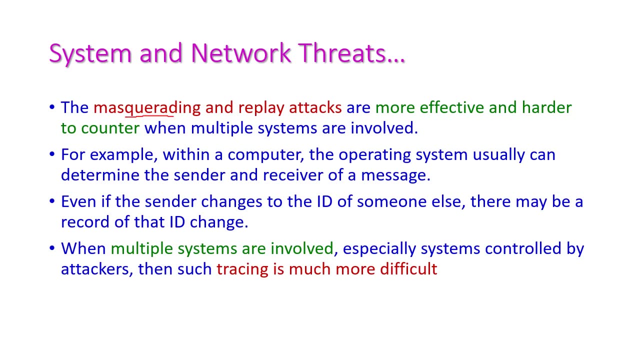 The ERP cases are important and different in terms of competence and skills. So when We talk about этомуutation, which is by the government lines, The ER P, Entonces estamos COMING до. Suppose if it is a single computer, then the operating system will take the entire control and if the sender changes its ID of someone else, then the OIS can easily identify and that will record the changes. 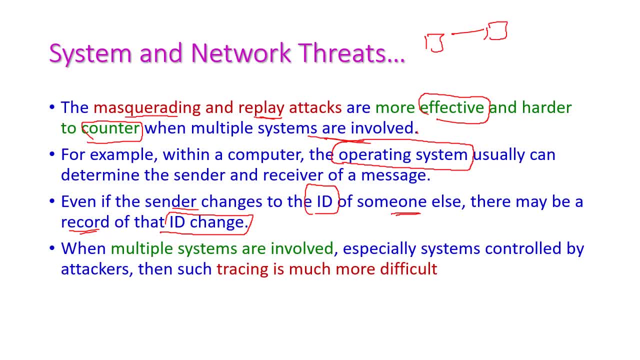 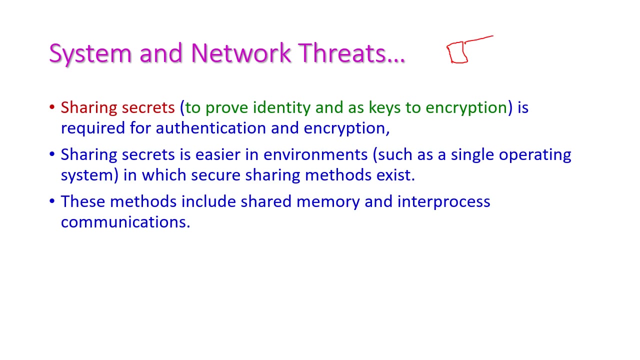 Okay, but when more computers are involved or connected to the network, then suppose if this network come under the control of attacker, then tracing of this particular changing ID is very, very difficult In the network. that is, more number of systems will be connected in the network. 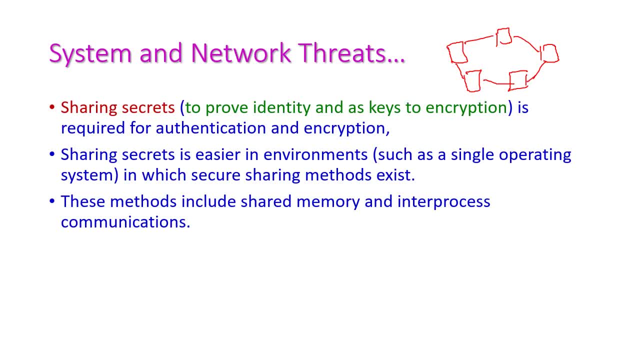 Then these systems will be communicated to each other Through message bossing, and through messages they can share the secrets, Okay, and the message will be first encrypted by using a secret key. Then the encrypted message will be transmitted from one place to the another place, that is, sender to receiver. 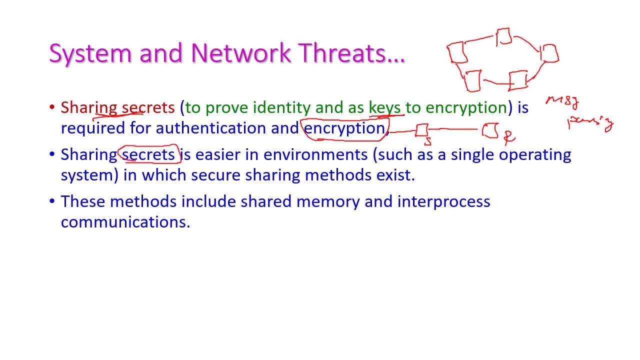 Right, and the sharing secret is easier in the environment, That is, if entire system is using only single operating system. Okay, and we can easily implement the secure sharing method so that we can easily keep the secret safe. right, and these methods include sharing memory and inter process communication. when the network is, the system should be connected with different networks. with different network, then this environment will be very, very difficult. 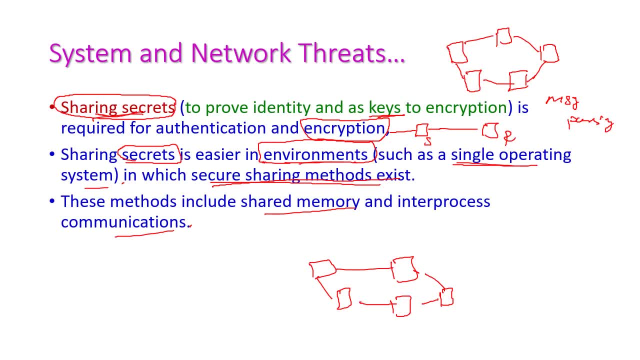 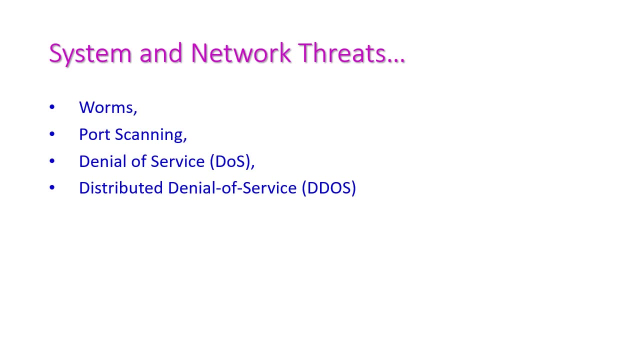 Okay, Okay, very difficult environment, So we have to protect our message secretly. then in this environment we will face lot of challenges. The most important challenges we are facing here is, that is, in the network and system. threats are the worms, port scanning, denial of service and distributed denial of service. 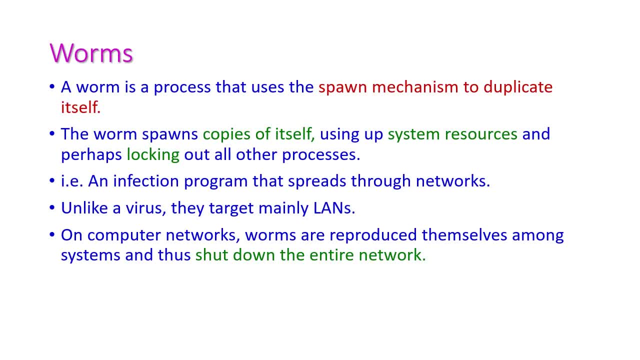 Let us see all those things one by one. The first one is worms. It is a process. It is a process That uses spawn mechanism to duplicate by itself, That is, the worms will copied, make a copies of itself by using the system resources. 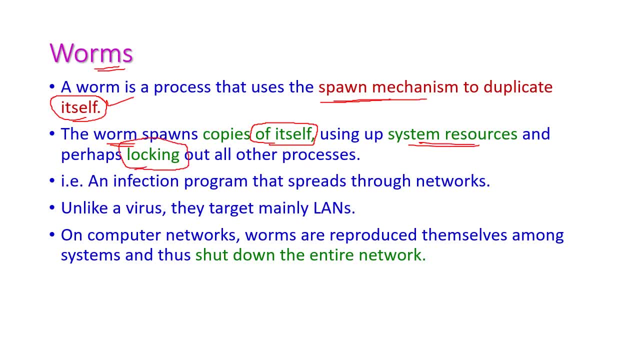 Hence it will lock out all the process on the computer processes. That means the infected program will spread throughout the network, throughout the network. Hence its main focus is to attack the local area network. Land means local area network. Okay, On computer networks the worms are reproduced themselves among the system that shut down the entire network. 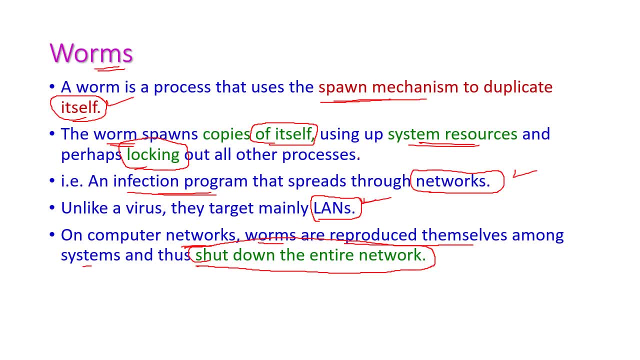 Okay, That is the same file will be copied more number of times, multiple times. Hence it will occupy all the CPU time as well as the main memory, Hence the entire network will be shut down. The worm actually attack the target system. 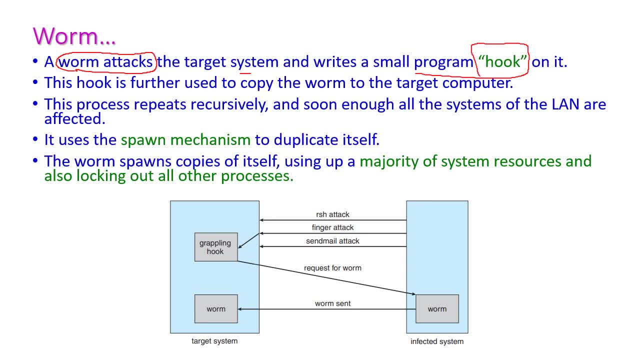 By writing a small program that will hook on it. Okay, This is our target system. from the infected system, The attacker will send this hook program to the target system. The user of this particular target system tries to download any of the file which are attached. these things: 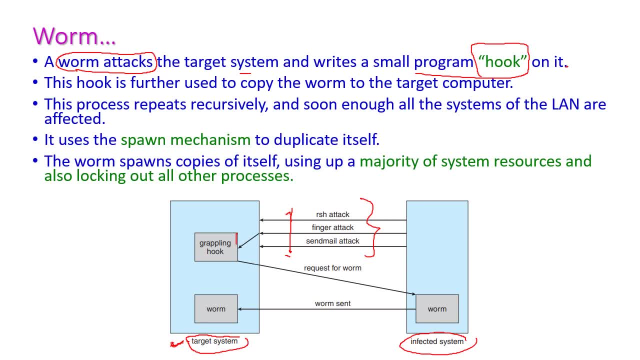 Once the user downloads the program then the hook will be attached to it. So without the knowledge of the user of target system, The hook will be copied into the target system Right. Once the hook copied here, it will send request to the infected system for this worm. 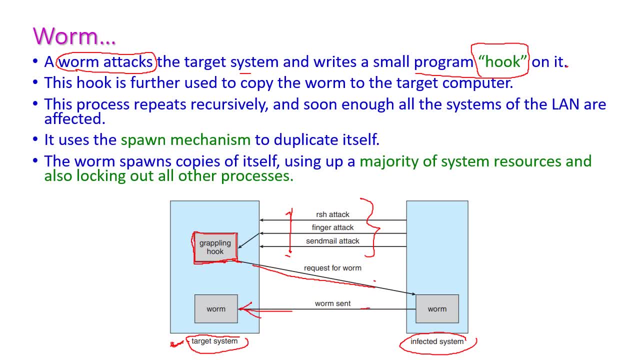 Then the worm will be copied to the target system Right Once the worm is copied here, then it will copy. It will make multiple copies of itself. Hence the system resources will be fully occupied by the worm And The entire system will get shut down. 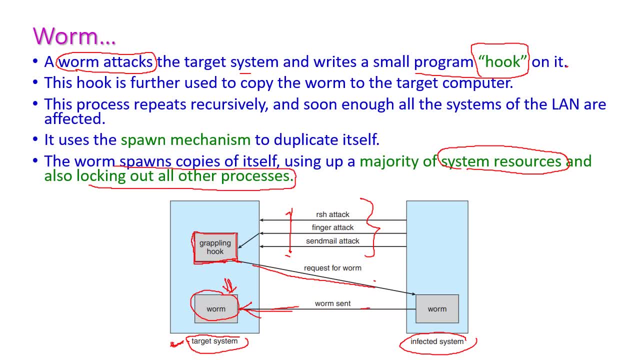 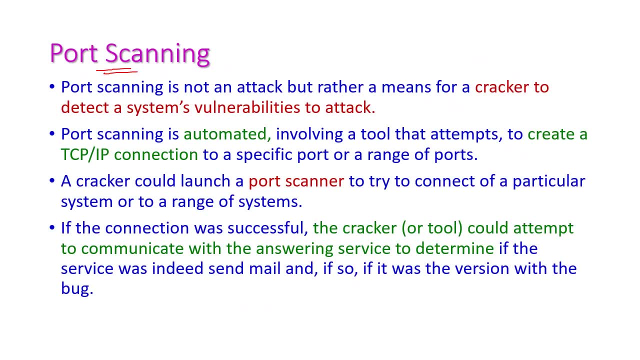 That is, it will lock out all the other processes of the entire network. Hence the entire network will be shut down. The next one is port scanning. It is not actually attack, But It crack to detect the systems vulnerabilities, to attack. Okay. 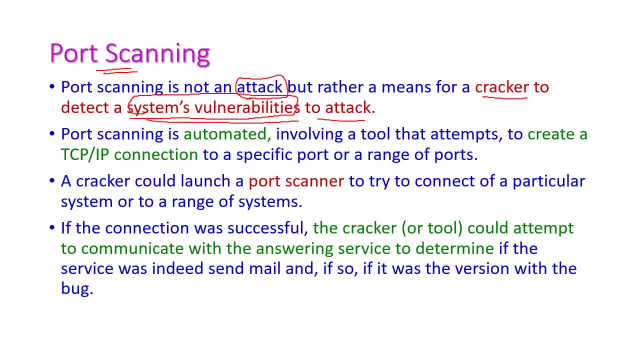 Systems vulnerabilities should be taken care. Okay, That is, The systems will be connected to the internet. Okay, And Those are communicating to each other. Okay, The port scanning is actually automated, Which involving tool to attempt create a TCP IP connection to specific port or range a port. 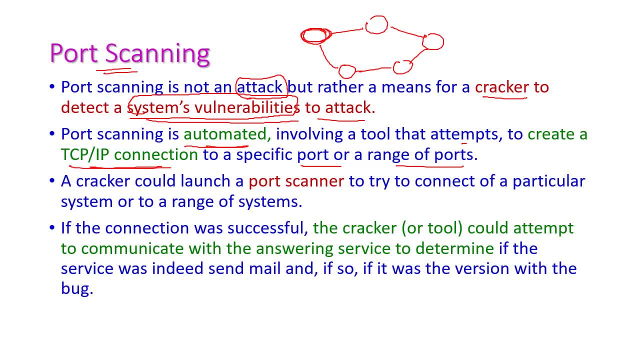 Suppose, if this is the system And the attacker try to collect the information- that is secret information- from this system, That Who are the other persons are in the network and they are sharing the information, the information, the secret information. okay, here the cracker could launch the port scanner. 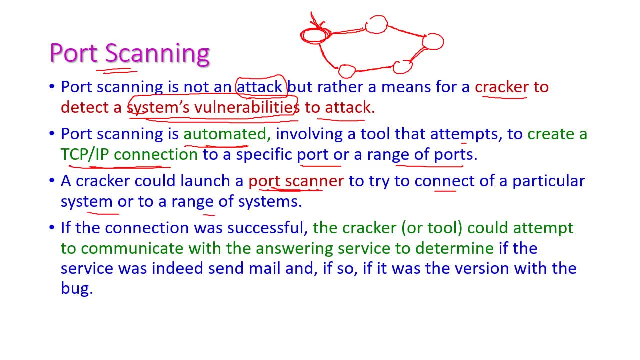 try to connect a particular system or range of system. okay, from here they will scan the entire network. okay, if connection was successful, then the cracker could attempt to communicate with the answering service. okay, if the service was sent mail. so it was the version with the bug. 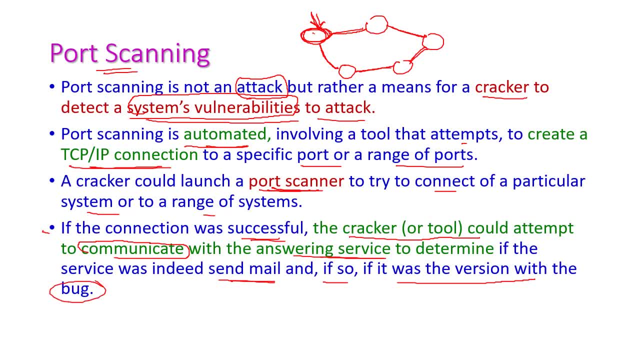 that means see instead of this particular person that is in this particular system um the attacker. they will send the message to all the other persons in the network instead of this particular person on this id. this particular system will send them message and they will collect the response also. 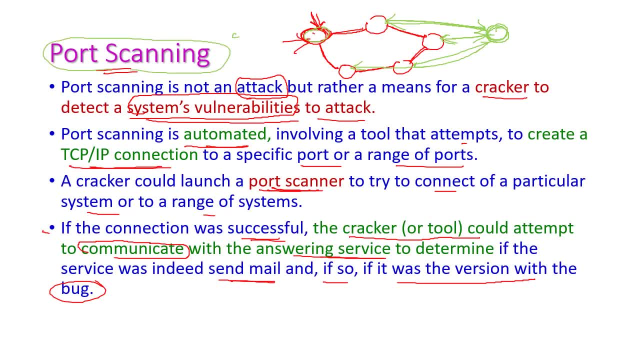 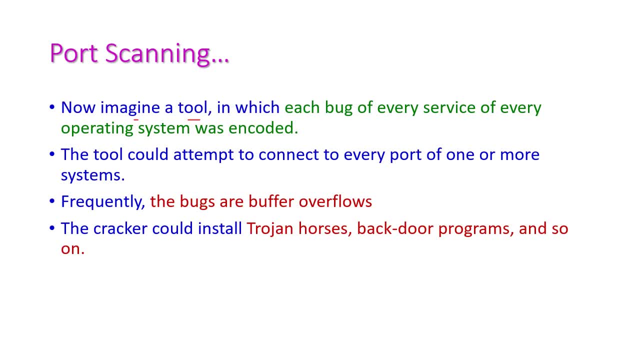 from all these things. so this is called as the port scanning. and now imagine this particular tool in which each bug of every service, of every operating system was encoded, that is, all the systems which are connected in the network will come under the control of attacker. okay, then the tool could. 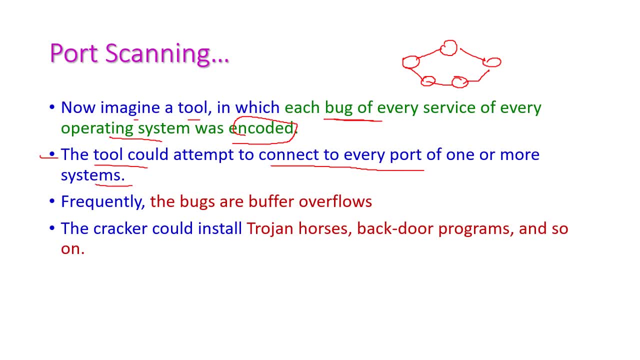 attempt to connect every port of one or more systems and the bugs are buffer overflows. okay, they can easily install, that is, the attacker can easily install Trojan horse, backdoor programs and so on on all the systems which are connected in the internet. right? the next important one is the denial of service, which is otherwise called as: 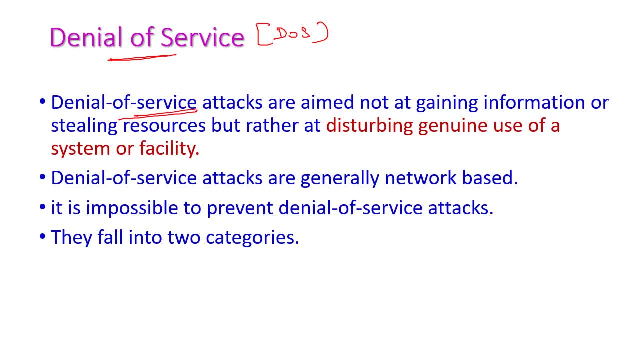 DOS. okay, the main aim of DOS is disturbing the genuine service of our system or the genuine facility of the system, and they are not interested in gaining information or stealing the system resources. okay, and this denial of service are generally a network based attack and it is impossible to 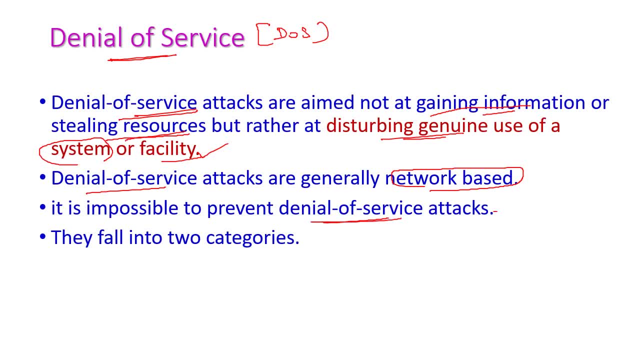 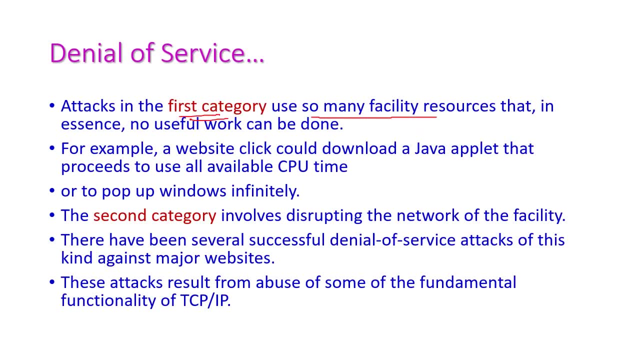 prevent this denial of service attack. they are other two categories. in this first category, the attacker will utilize the system resources and, finally, there is no useful work will be done. okay, that is, if we click any of the website, that will download the Java Upload. that is, we are not actually in need of this particular Java Upload. 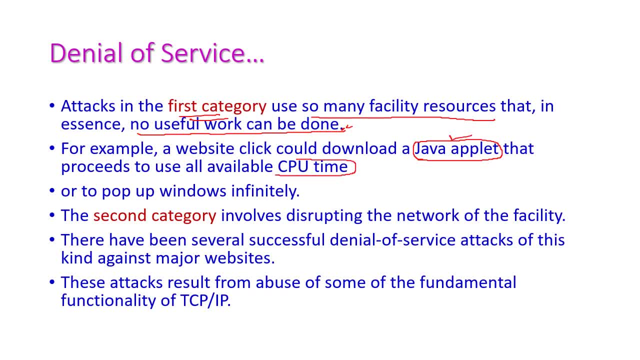 blood. hence it will utilize all the cpu time and our work will be disturbed. okay, otherwise some pop-up window will be displayed. our monitor continuously, infinitive time the pop-up window will be displayed. so this will this disturb our normal work? when come to second category, it 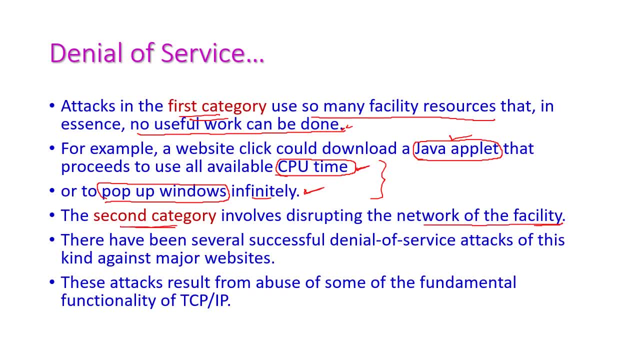 involves disturbing the network of the facility. okay, that is a several successful denial of service attacks in this kind of major websites. okay, they will continuously disturb our normal work and these attacks results from abuse of some fundamental functionality of tcp. the next one is distributed denial of service. 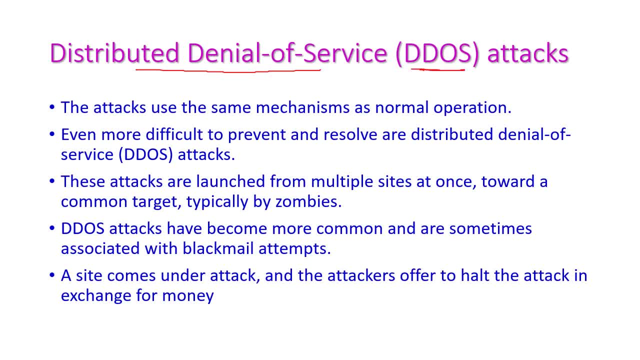 attack, which is otherwise called as ddos, and this attack is even more difficult to prevent, and this is very dangerous one when compared to distributed, that is, denial of service. okay, these attacks are launched from multiple sites at one. okay, the system which are connected to a single. 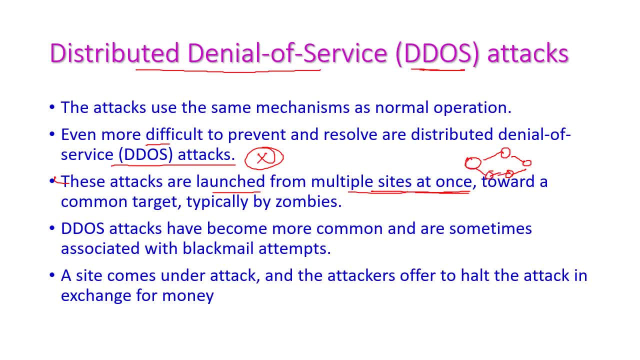 system, that is, target system from this, all the connected systems will be affected by this distributed denial of service. okay, that is, the attack will be launched at multiple sites at one towards a common target, typically a zombies. okay, this attack have become more common under sometimes associated with: